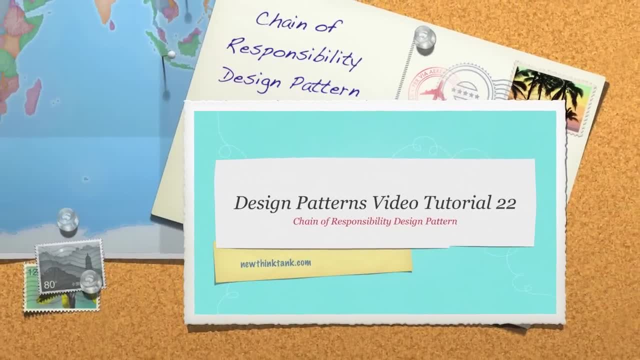 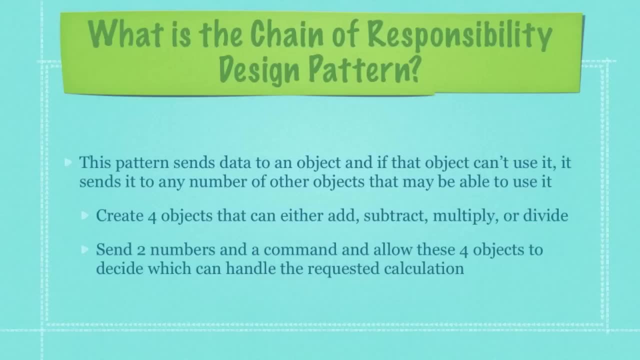 Well, hello internet and welcome to part 22 of my design patterns video tutorial. Today, we're going to talk about the chain of responsibility design pattern. So what exactly is the chain of responsibility design pattern? Well, this pattern has a group of objects that are expected to 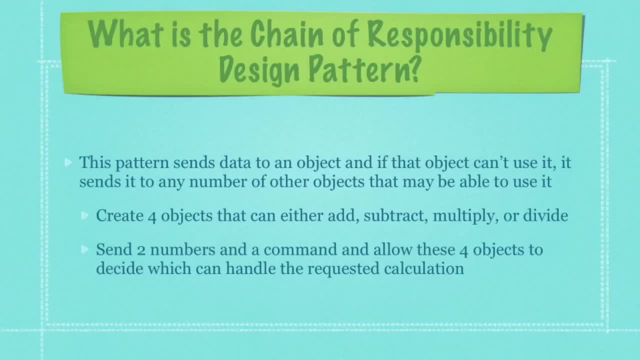 between them be able to solve a problem, and if the first object can't solve it, it just simply passes the data to the next object in the chain. In the example in this presentation, I'm going to create four objects that can either add, subtract, multiply or divide two numbers that are sent. What? 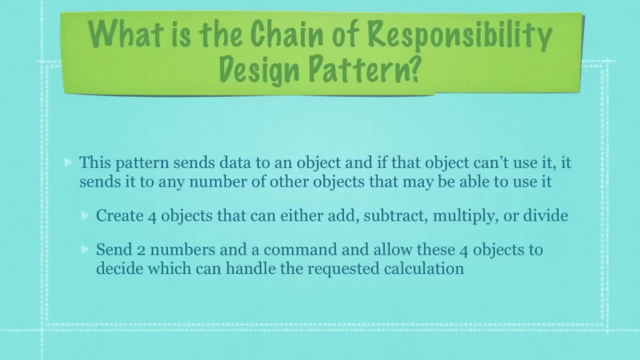 you're simply going to do here, or the client's going to do, is send two numbers in a command and allow these four objects to decide which can handle the requested calculation. So let's look at a UML diagram to sort this out. Basically, we have our client, just like always, and then, of course, we're 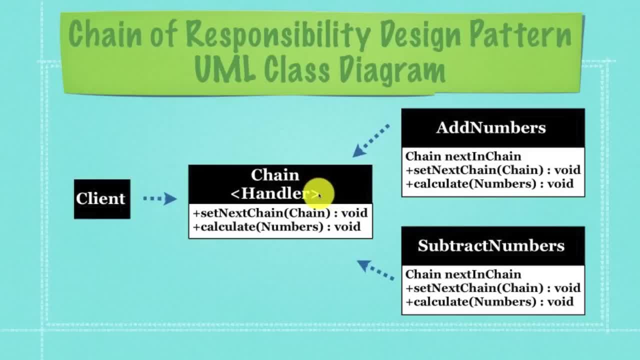 going to have a chain interface- and this is referred to as the handler- and inside of it we're going to have set next chain, Which is going to be passed a chain object. Now, what set next chain is going to do is it is going to be: 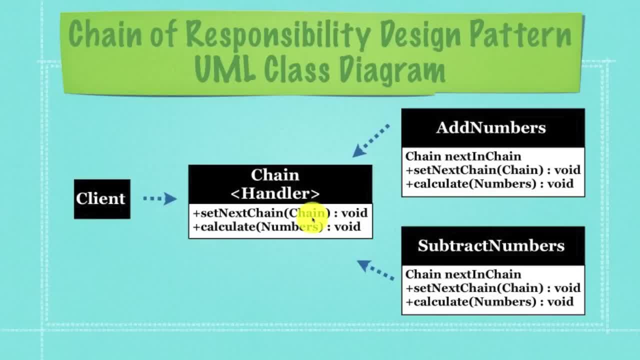 passed of reference to the next object to call in the chain. if it is needed, Then calculate, which is going to be implemented by both add numbers and subtract numbers, multiply numbers and divide numbers, which you're going to see here in a minute. What calculate is going to do is either make the 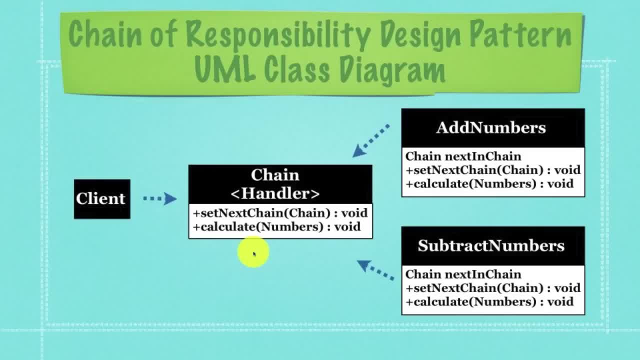 calculation or call the calculate method, on the next object set by this client. This guy right here Set next chain. So if it can't make the calculation- like add numbers down here can't make the calculation- it is going to say: OK, what is the next object in the chain which is going to be? 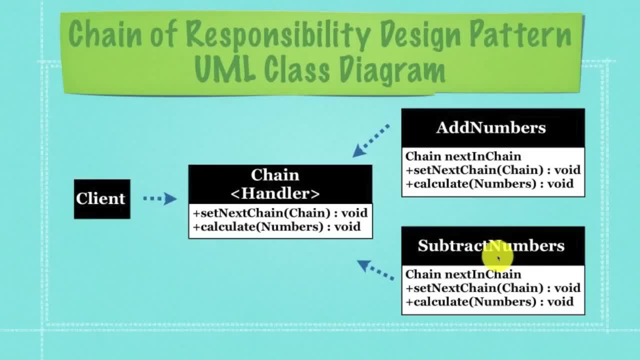 subtract numbers and it's going to say: OK, let's call calculate on subtract numbers based off of the fact that subtract numbers object is going to be stored by set next chain. That didn't make any sense. Don't worry about it. We're going to get into the code and go through this step by step. 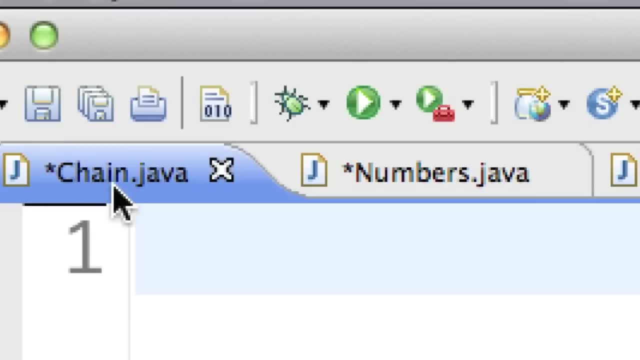 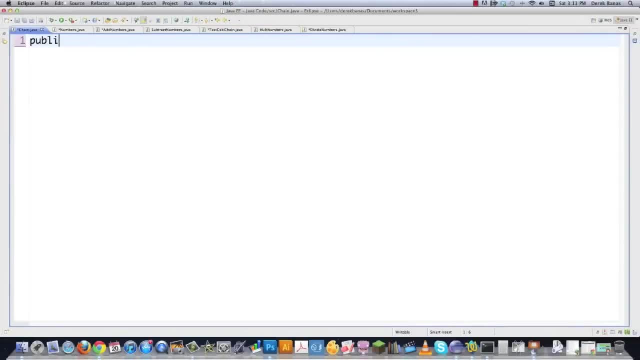 OK, So here I am, over in Eclipse and we're going to start writing some code. First thing we're going to do is create our interface called chain dot Java, So let's just go in here. This is very simple, Don't worry about it. 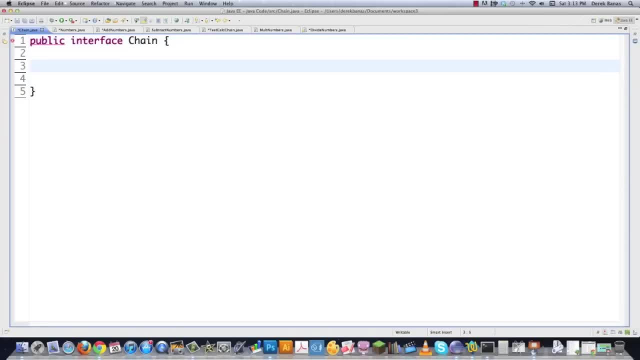 And it's an interface and I'm going to call it chain and it doesn't have to be called chain. I just thought it made sense that way. And then here we're going to define the next object to receive the data if this object is unable to process. 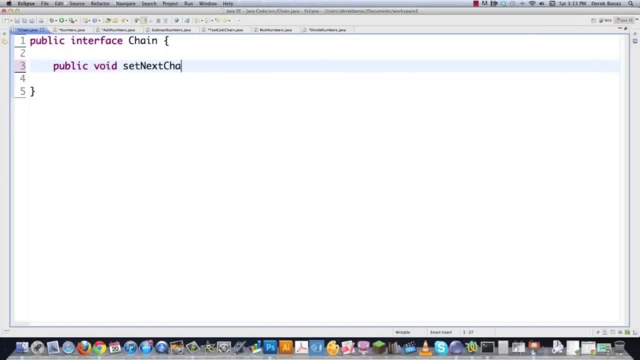 it. So when you go public void, set next chain and it's going to be passed an object that implements the chain in her Interface and we're just going to call it next chain because that seems to make sense. And then we're also going to 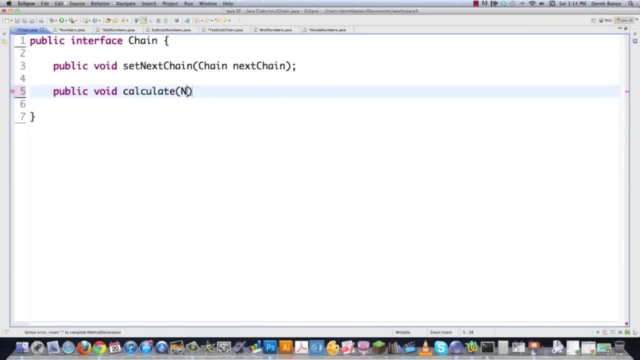 force it to make a calculation of some sort, And it's going to be passed a object called numbers, And here I'm just going to call it request, And that's it, You're done. There is the chain interface, So now let's jump over into a 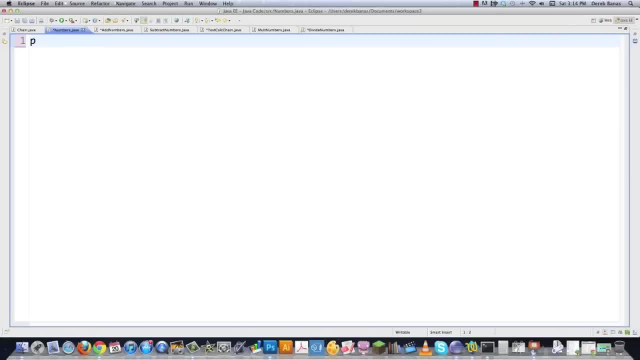 numbers, dot Java and see exactly what's being passed to it. So we're just going to go public class numbers and then we're going to store private int- Number one private and number two private string calculation wanted, And this is going to ultimately decide on which. 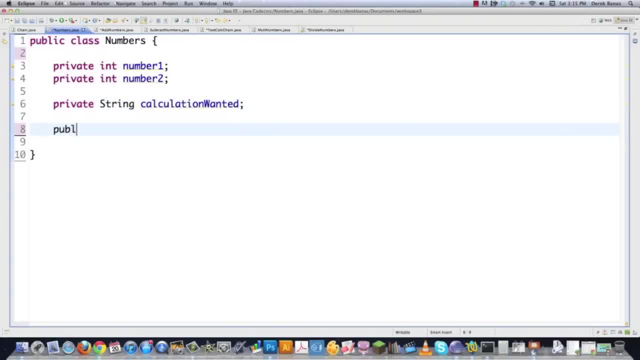 one of these calculate methods is going to be called in which object that implements the chain interface, And then numbers is going to be passed- new number one, new number two, as well as a string count wanted, And then it's just going to simply take all these guys. Number one: 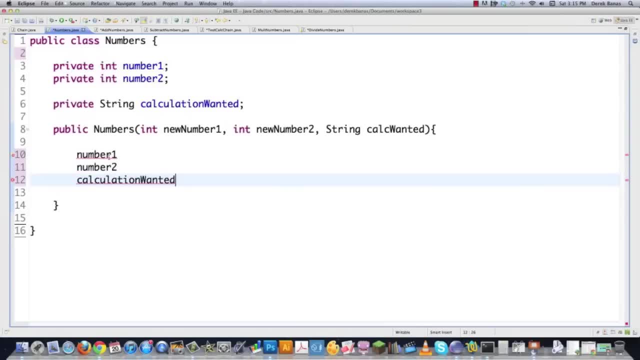 Number two, Number two and calculation wanted and store those inside of here. Real simple. I'll save that And then, if we want to be able to get access to these numbers, public int, get number one And it's just going to return number one, of course, And 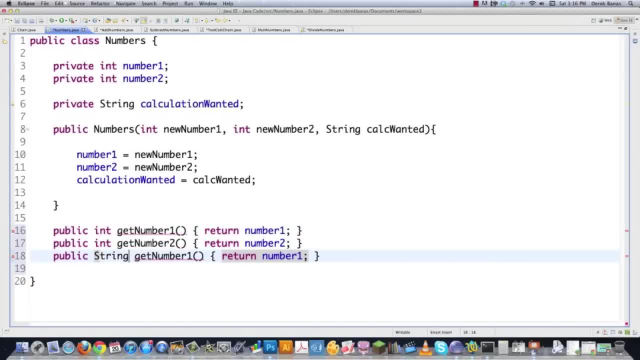 then this guy is going to return number two And then this is going to be a string: count wanted. And here we're going to return calculation wanted, File, save it, Ready to go. So now we're going to do add numbers And you're going to get to. 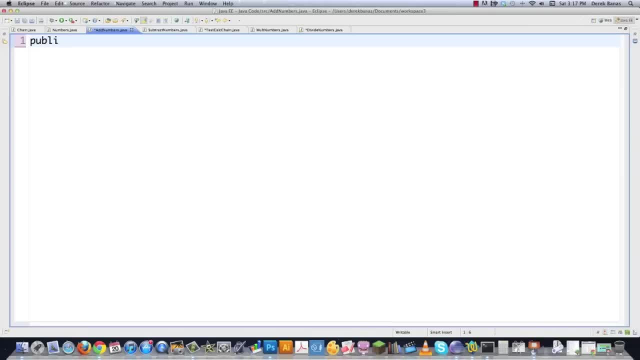 see how this is all put together. So this is going to be real simple. We're just going to go public class, add numbers, implements, chain, And then each one of these is going to store the next object in the chain that can perform these calculations. And here, in this constructor, we're 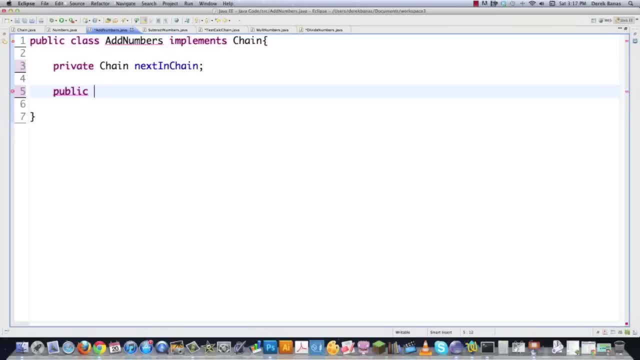 going to define that next object that's going to receive this data. If this object is unable to use it, Let's just go up to add numbers, Add on implemented methods, Save ourselves some time. And here we're just going to go next chain Or, in this situation, we'll go this: Next chain is equal to next chain. 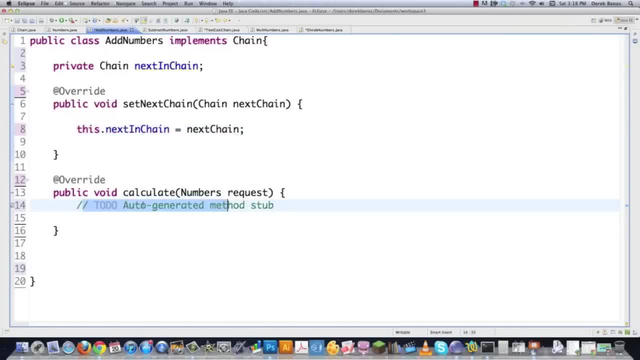 That works, And then down here in the calculation section, everything is going to be based off of a string. So we're going to get request, Get calc wanted And we're going to ask it if add is the name for that string And if it is just. 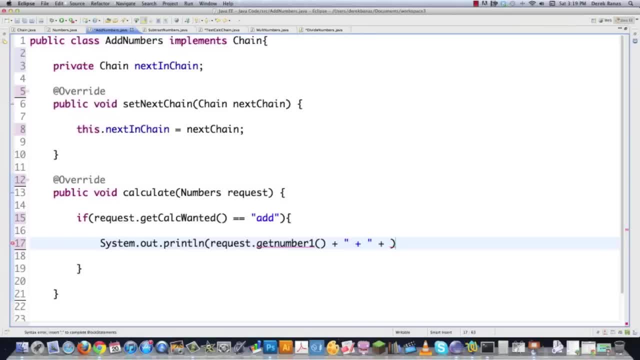 go request, Get number one, Plus Plus Number two, And this is just going to show them on the screen- Plus Equal sign, And then we can just take this and add these two numbers together. So it's a quick and dirty way to do it. 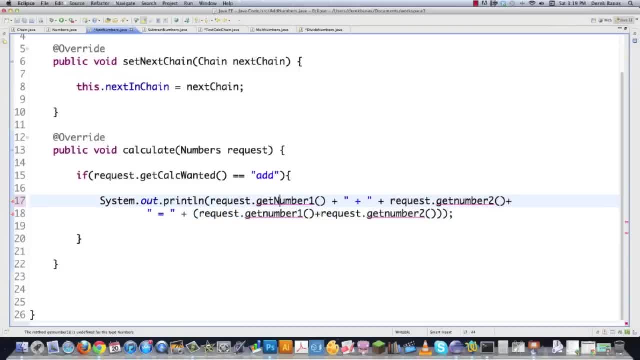 to get that information And that's just going to shoot it on the screen. This is going to be capitalized, of course. There we are, Else, if they did not send a string add like you see right here. Well, real simple, We're just going to. 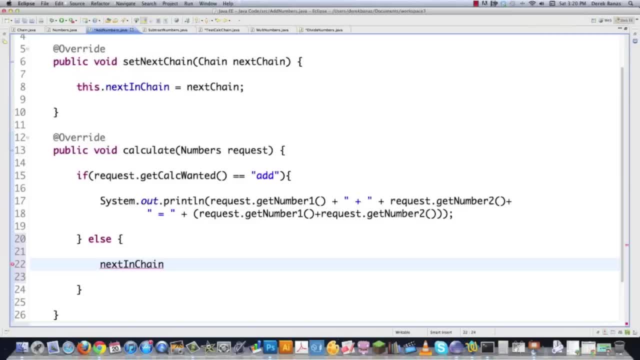 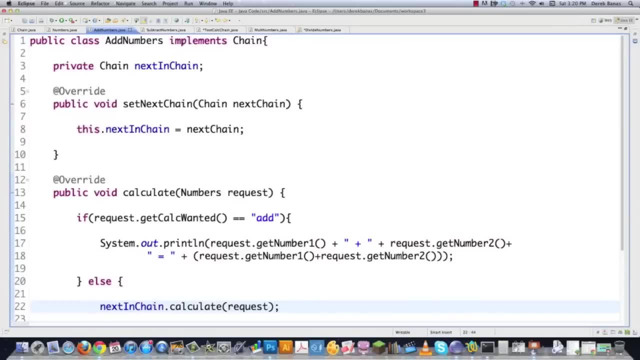 say: well, I'm not going to worry about it, Let's let the next object in the chain calculate it Or figure it out, And we're just going to pass them that number object called request, File save And you're going to see the only thing. 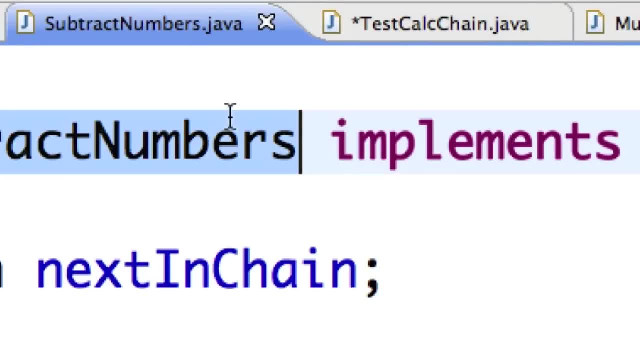 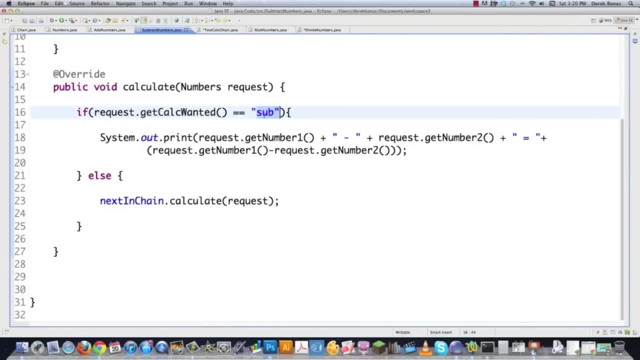 that's really going to change is: let's go into subtract numbers right here And you can see. everything is exactly the same just like before. The only difference is: here we're going to check to see if sub was passed along, And here we're going to subtract from it, And then you're also going to see the same thing is. 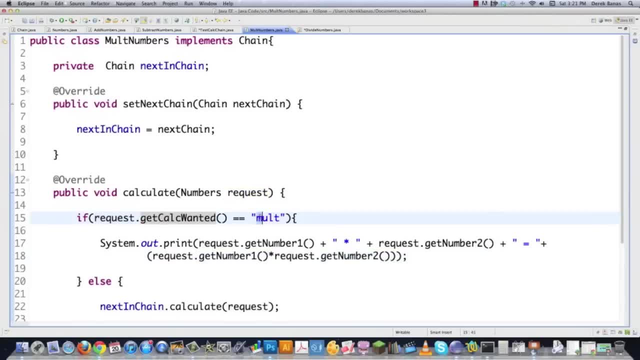 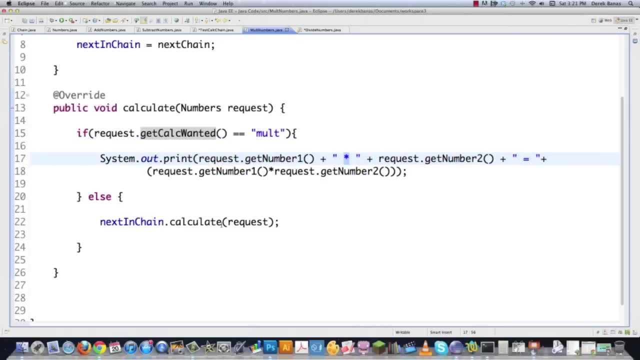 going to be true for malt numbers. There you can see, malt is being passed over, And here we're doing a multiplication instead of subtractions or additions. And then I'm going to go into divide numbers, dot Java and actually do this all from the beginning. 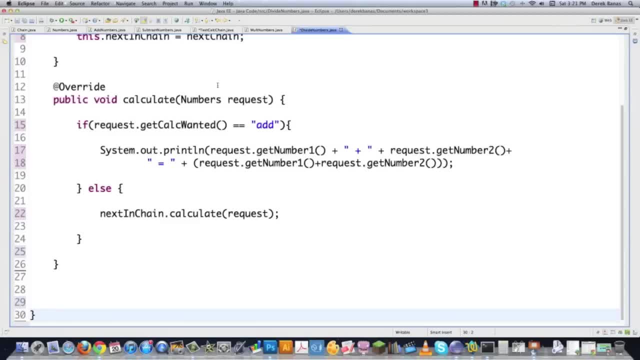 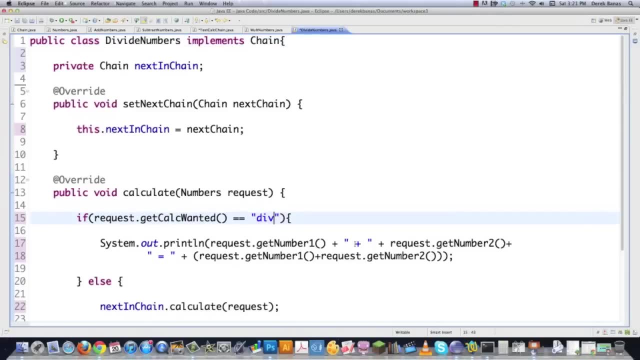 Except I'm just going to copy this, because not much is going to change either, Even though this is a completely different one: Divide numbers. all the same, The only thing is we're going to type in here, div, And here we're going to put in a division sign And here: 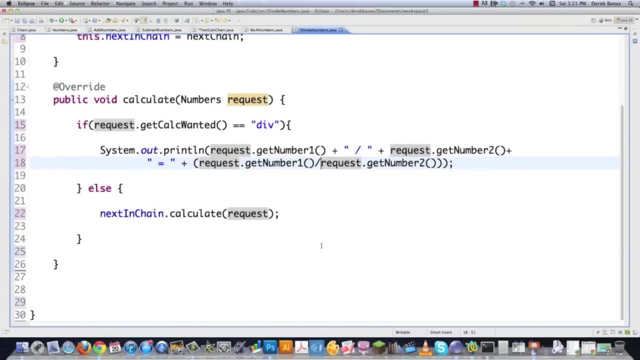 we're going to put in a division sign, So that's going to handle those divisions, And then down here else, what we can do is print out a command. I mean, this is just the basics of how this works. You can use this for numerous different things. It's basically 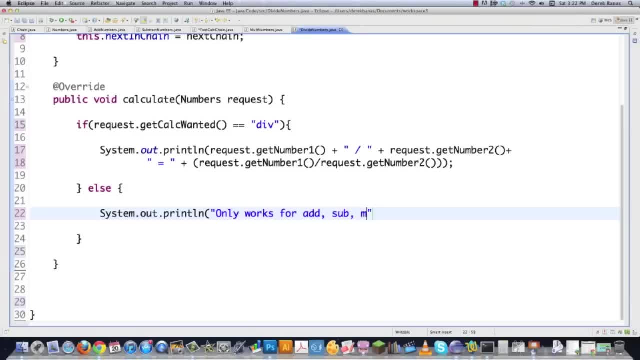 just how to pass the buck to other objects, as the whole entire idea of using this pattern, Which is very, very useful. And here we are. we can print out an error message if none of those other things work, Alright. So there we are, we're done. 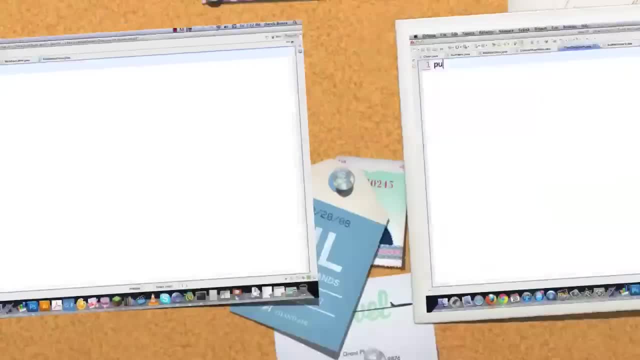 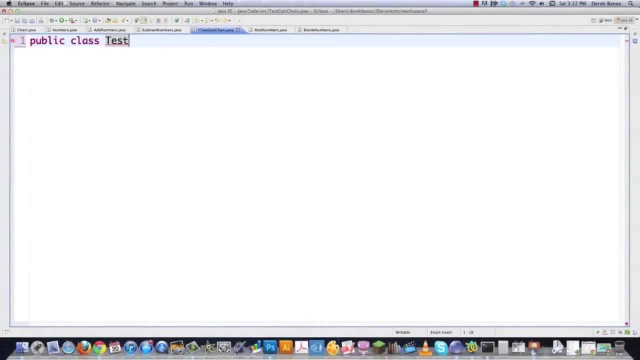 Let's jump in here and test this guy. So let's go test calc chain And this is going to be public and all the code is available underneath the video. If you want to really learn this stuff, go get it Heavily commented to help you understand. 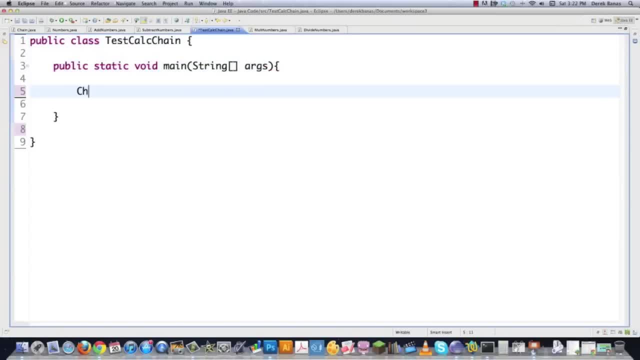 what's going on here And here we are ARCS, And then what we're going to do is create our chain objects. So calc1 is going to equal to new add numbers. This is really where all the magic happens, And then we need to do this for all of our potential calculation objects: calc2,, calc3,. 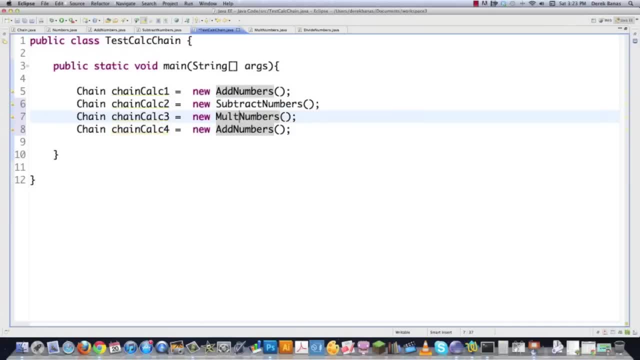 and calc4.. And then this is going to be subtract, mult and divide. So there we are. We have all those set up inside of here, And then next I'm going to tell each object where to forward the data if it can't process. 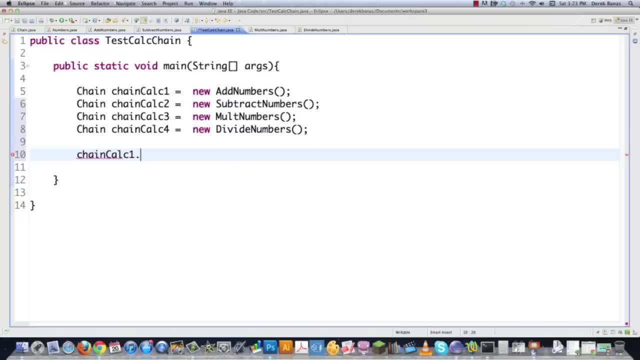 the request. So we're going to go chain calc1, set next chain which is in every single one of these objects that implement the chain interface like that, And then we're going to do that for three of these guys, so the second one and the third. 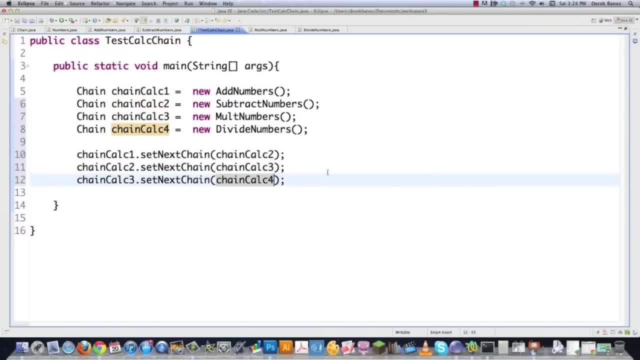 one, And then this is just going to be three, and this is going to be four, And that's just going to pass everything to the right place, And then we're just going to define the data in the number objects and send it to the first. 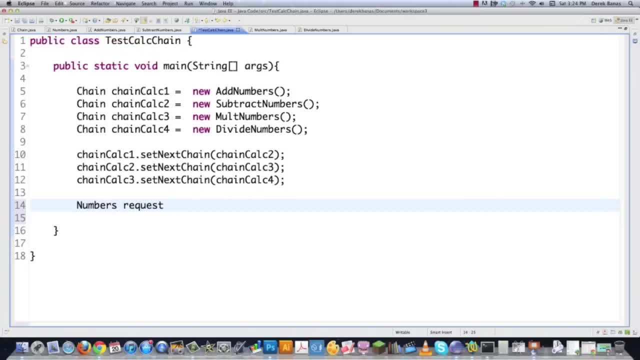 object in the chain. So just go numbers. request is equal to new Numbers and let's say we want to pass it a 4,, a 2, and add, I'll save, And then we're just going to go chain calc1, which is the beginning of our chain, to find. 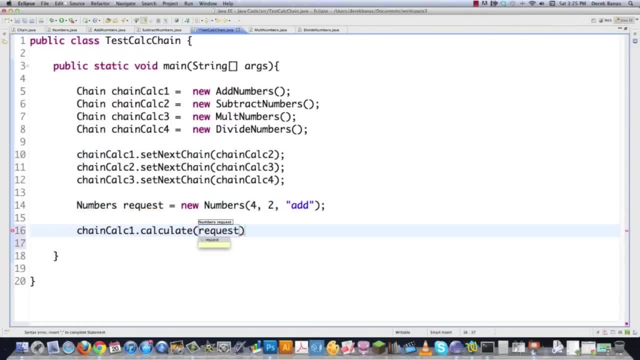 that And pass request, which is the numbers. object to it and let it do its job. That's it. Execute, see what happens. And there you can see 4 plus 2 is equal to 6. And just as easily let's go multiply. didn't really have to change anything. execute it. 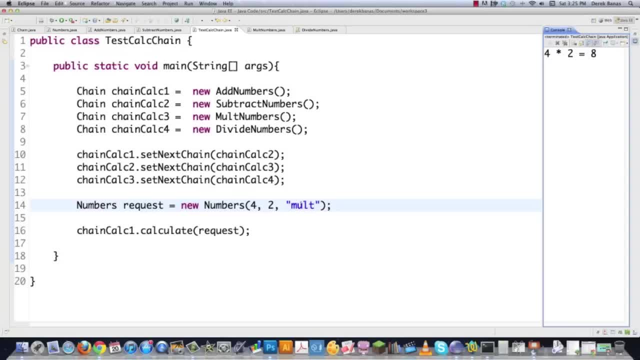 again, 4 times 2 is equal to 8.. And what happens if we would do something like type in: pow, I'll save, execute, And there you go. You get a little bit of an error message. Only works for add, subtract, multiply and divide.